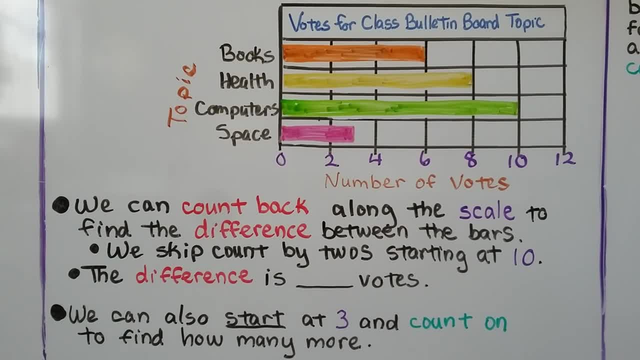 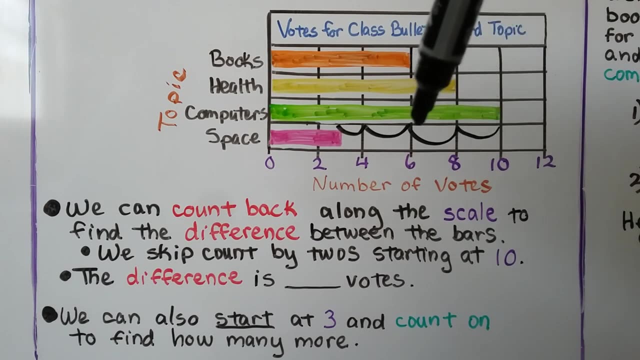 We can count back along the scale to find the difference between the bars. We can skip count by twos, starting at the ten. We skip count starting at the ten. Two, four, six and one more would be seven. The difference is seven votes. We could also start at the three for space. 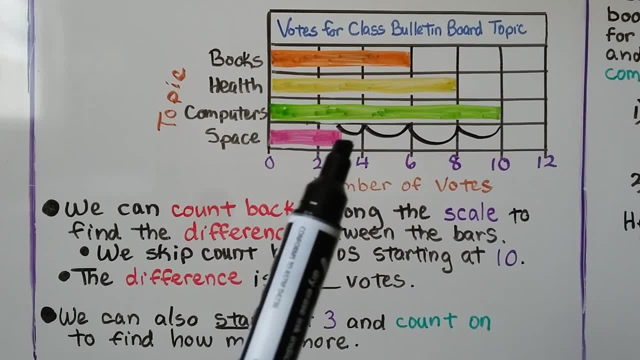 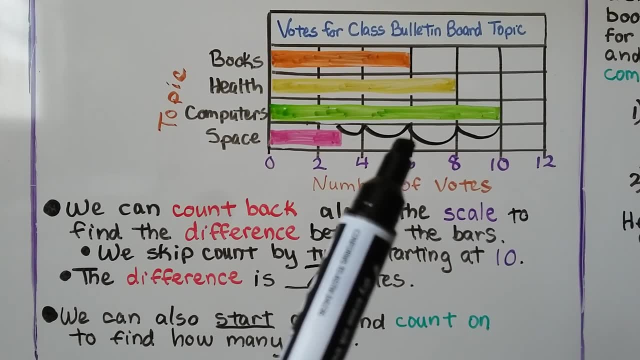 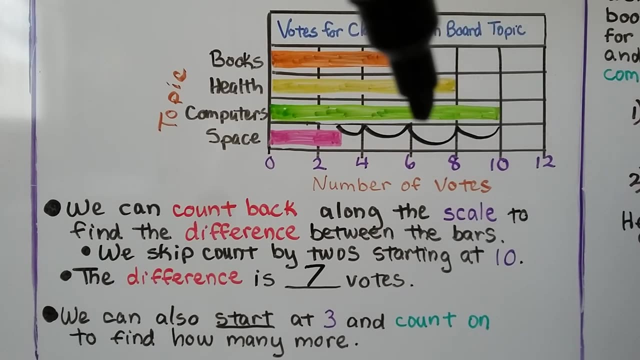 and count on to find how many more. Three and going to four would be one plus two more two is three and two more is five and two more is seven. but it's a lot easier to skip count coming back, isn't it? And then adding the one more between the four and. 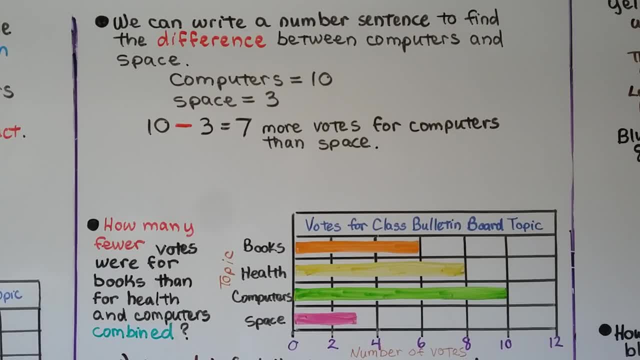 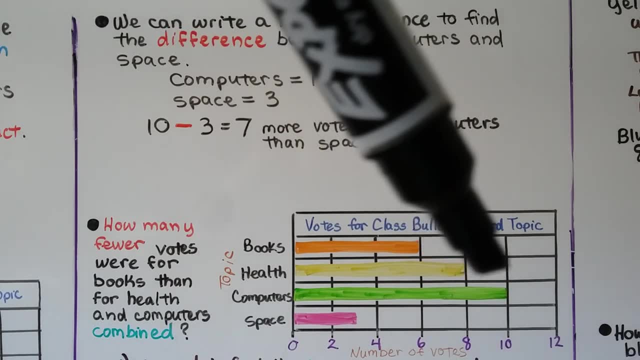 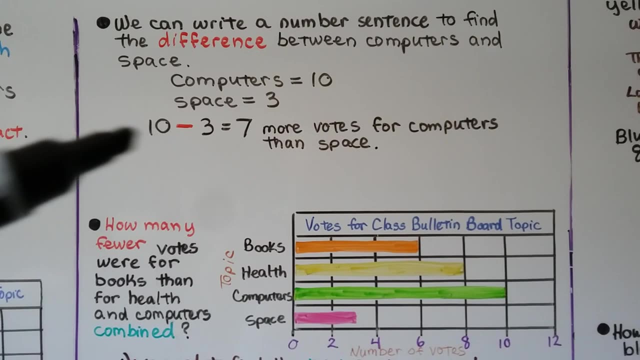 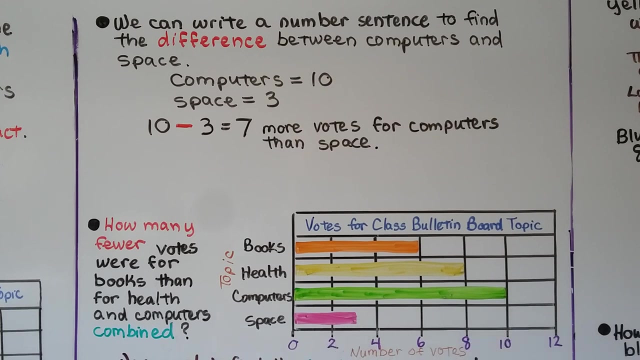 three. We could also write a number sentence to find the difference between computers and space. Computers is ten and space is three. We can do ten Minus 3 is equal to 7, so we know 7 more votes were for computers than space. 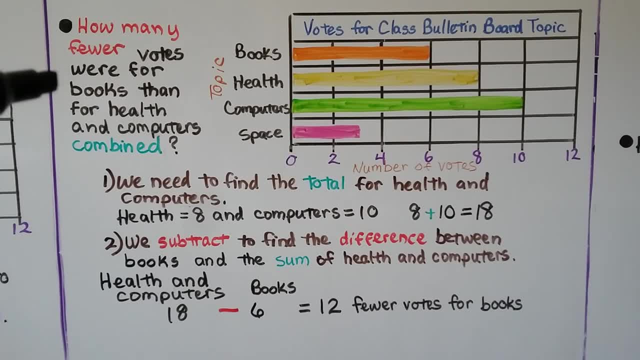 How many fewer votes were for books than for health and computers combined. The first thing we need to do is find the total for health and computers. It wants health and computers combined. Health is 8.. Computers is 10.. 8,- 10.. We add them 8 plus 10. 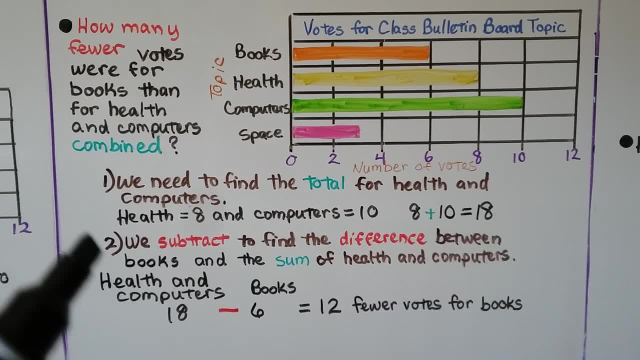 is equal to 18.. Now we need to find the difference between 18 and the number of books. We subtract to find the difference between books and the sum of health and computers. Health and computers is 18.. Books is 6.. We do 18 minus 6.. 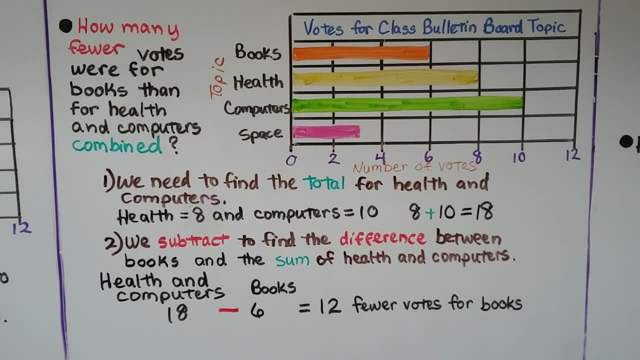 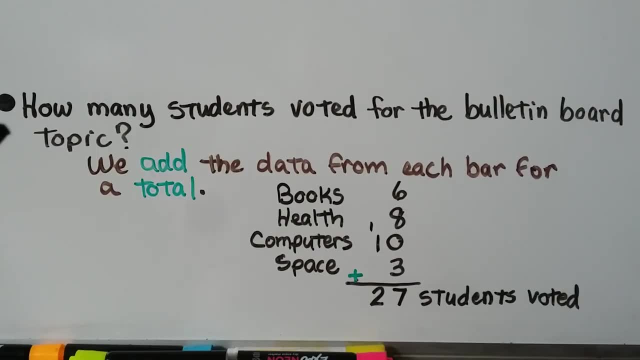 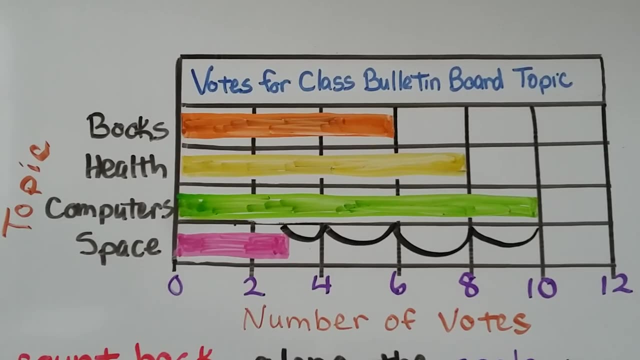 6 is equal to 12.. Fewer votes for books. How many students voted for the bulletin board topic? We add the data from each bar. for a total, We need to add 6 plus 8 plus 10 plus 3.. 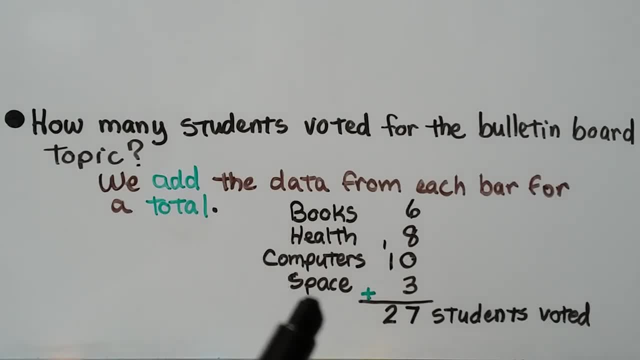 6 books, 8 health, 10 computers, 3 space. We start in the ones column 8 plus 6 is 14, plus 3 more is 17.. That's 1, 10 and 7 ones. We regroup the 10 to the tens place and put the 7 in the ones place. We add 1 plus 1 for the tens. 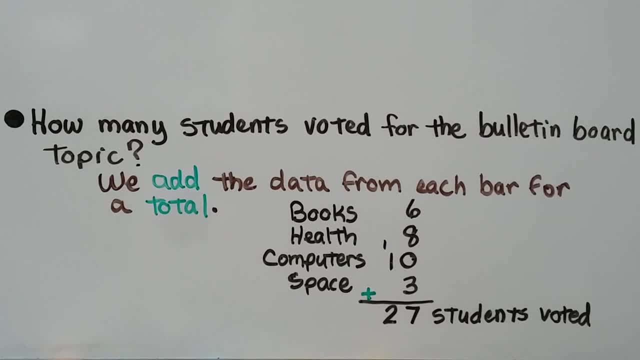 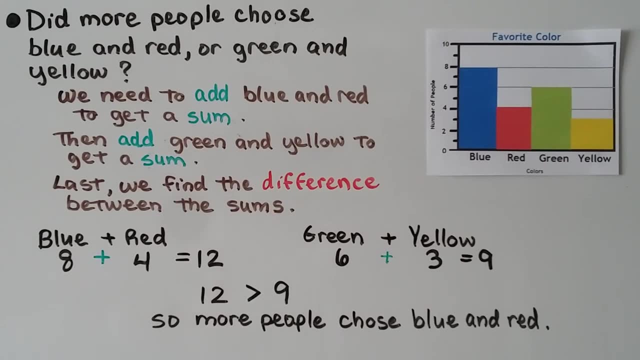 We get 27 students voted. Here we have our bar graph about favorite colors. Did more people choose blue and red or green and yellow? That means we need to add blue and red to get a sum, then add green and yellow to get a sum. Let's take a look at the graph. 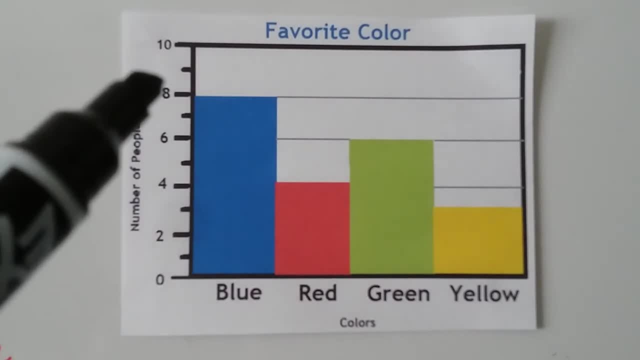 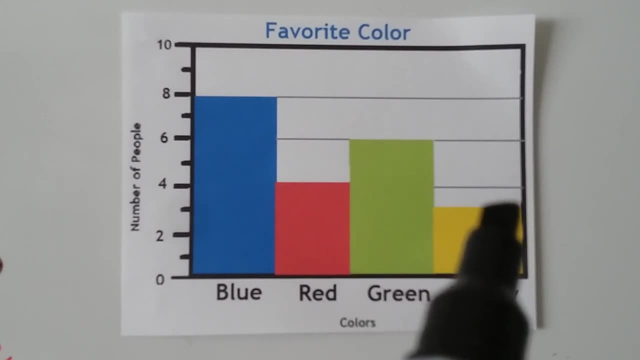 We need to add blue and red, so we're going to need to add 8 and 4.. Then we're going to need to add green and yellow, so we need to add a 6 and a 3.. In between the 2 and 4, it must be 3.. We need 8 plus 4, then we need 6 plus 3.. 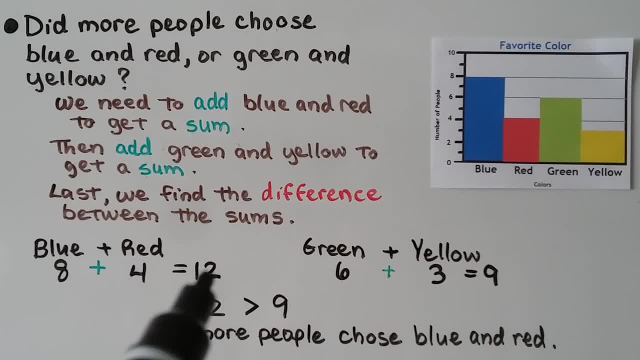 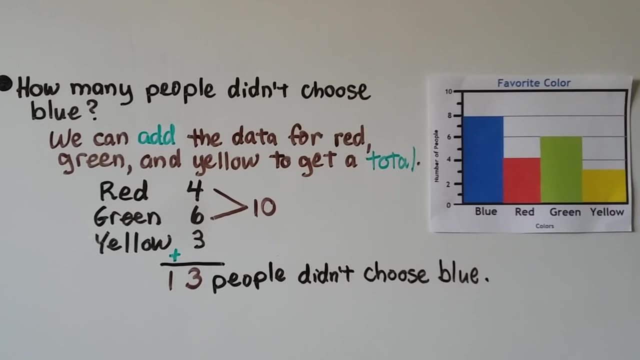 8 blue and 4 red is equal to 12, and 6 green and 3 yellow is equal to 9.. 12 is greater than 9, so more people chose blue and red. We will also find out what student was chosen. 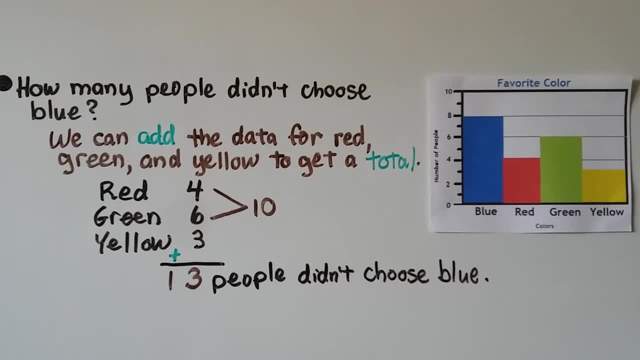 How many people didn't choose blue. We can add the data for red, green and yellow to get a total. Red is four, green is six, yellow is three. We do four plus six plus three. Four plus six is 10.. 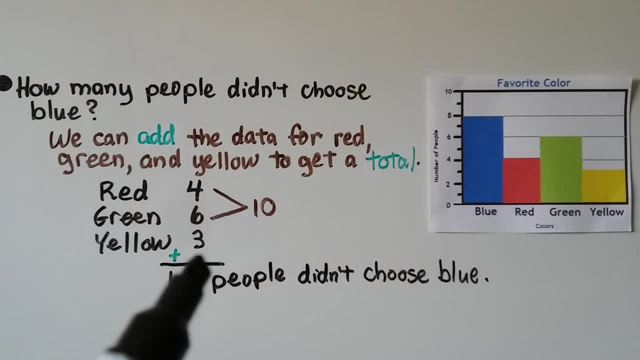 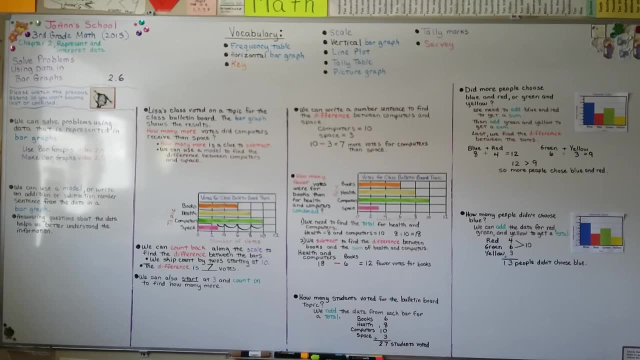 They're friendly numbers because they make a 10. Then we can do 10 plus three. We know it's 13. people didn't choose blue, So we can solve problems using the data, the information in bar graphs, and we can use a model or write an addition. 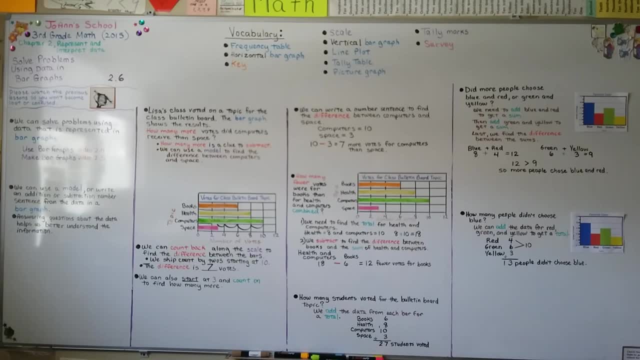 or subtraction number sentence and answer questions about the information. We can use the scale to help us skip, count back or forward, to compare the bars and the totals. We can even find the total of all of the numbers by finding the total of the numbers for the bars.